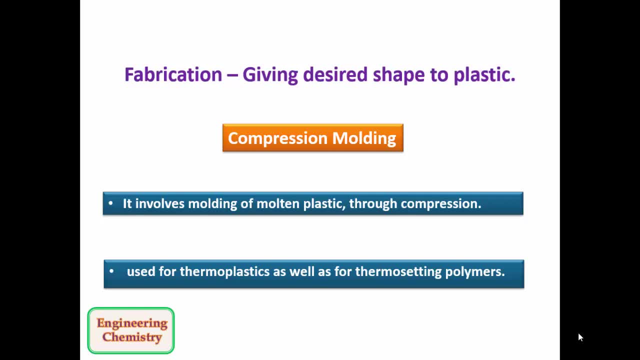 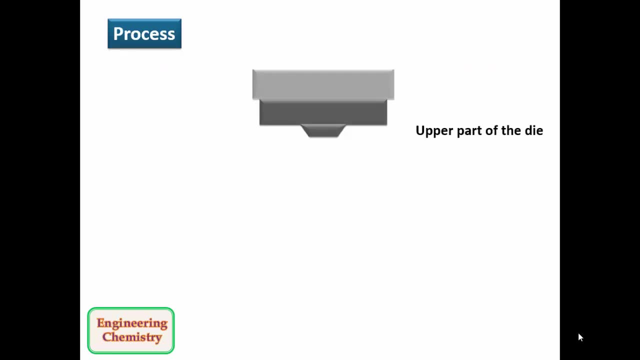 used for the thermoplastic as well as for thermosetting polymers. Let us understand the process of compression molding. It consists of two parts: upper part of the die and lower part of the die. The lower part of the die is fixed and upper part of the die is movable through guide. 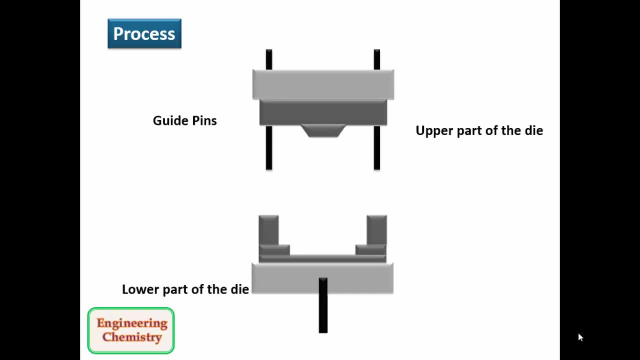 pins. Lower part of the die has the facility of heating as well as cooling Predetermined quantities of plastic materials. Then the two halves are closed by applying the pressure. Here the pressure is about 100 to 500 kilogram per centimeter square, and then the article is heated at around 130 to 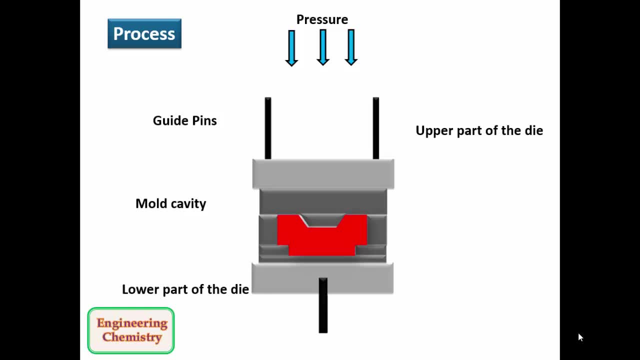 180 degree Celsius. Finally, the curing time is about 20 to 30 minutes. The curing is done. Curing means heating in the case of thermosetting polymers and cooling in the case of thermoplastic polymers. This is because, in case of thermoplastic polymers, 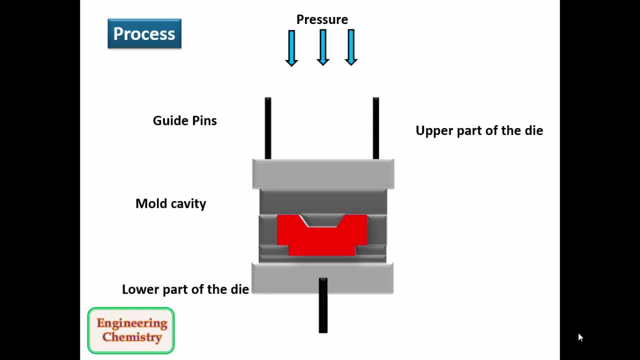 it is just a addition, polymerization, and it is a exothermic reaction. Hence, to take the reaction into the forward direction, we need cooling, Whereas in the case of thermosetting polymer, it is a condensation reaction in which small, simple molecules like H2O, NH3 are. 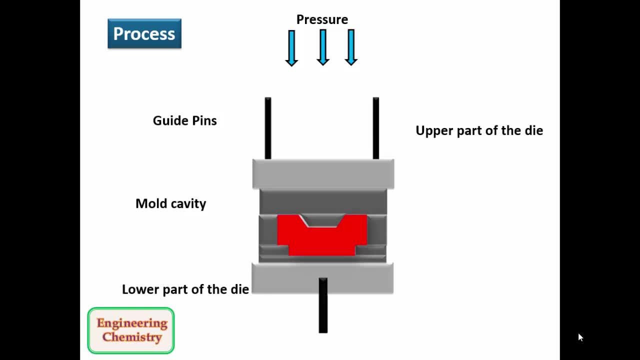 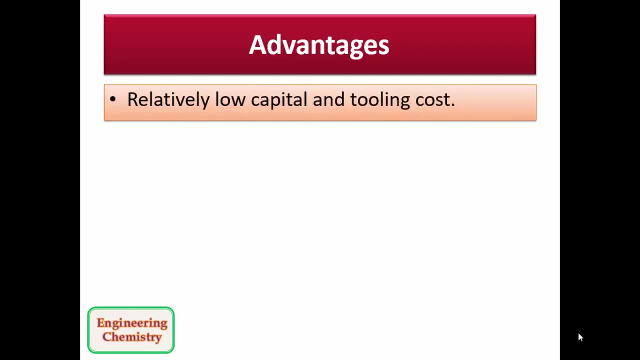 eliminated and hence to eliminate these molecules we require heating. Finally, with the help of extraction pin, the molds are opened and the article is taken out. Let us see the advantages of compression molding. It requires relatively low capital and tooling cost, low mold maintenance. The product has low residual stress and products retains mechanical 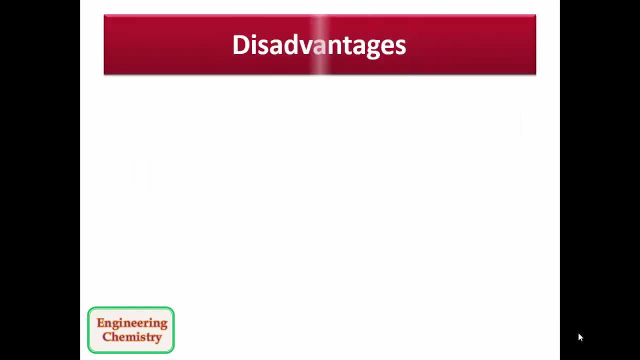 and electrical properties. However, it is a very efficient mold remover. It is a very efficient mold remover. It is a very efficient mold remover. It is a very efficient mold. however, it has some disadvantages. also, it is not economical for making a small number of parts. 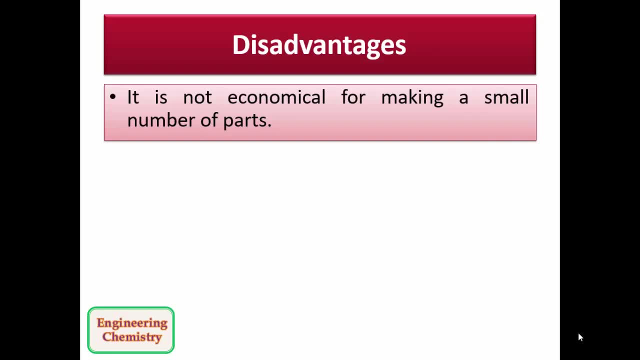 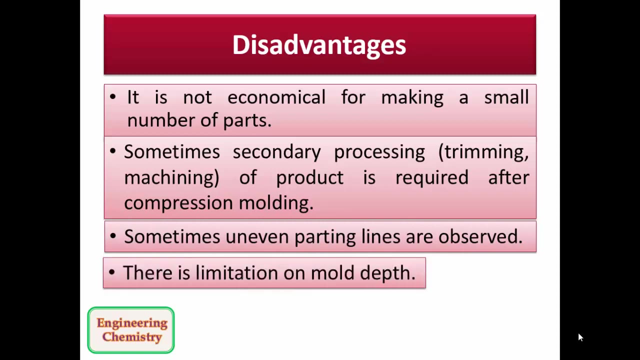 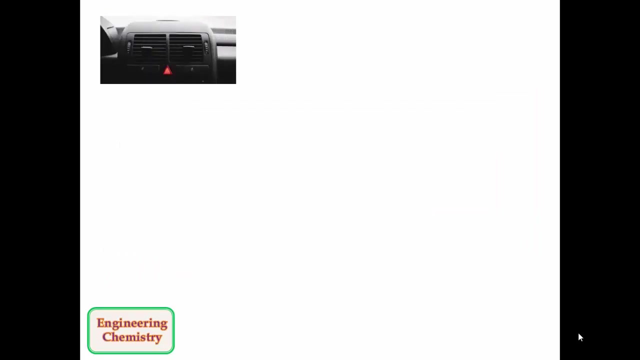 that means once the molds are manufactured, it should be used for for large number of parts of same size. sometimes secondary processing of product is required. after compression molding, uneven parting lines are also observed and there is a limitation on mold depth. let us see the applications of compression molding. with the help of compression molding, we can make: